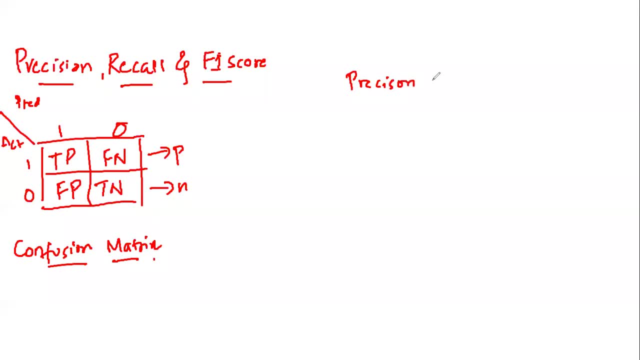 of this, precision and recall measures. So precision and recall are basically used for information retrieval. Now, in terms of information retrieval, the example that I would like to give you is basically Google search engine. In Google search engine, whenever you write a query, you basically are searching for something. Then, based on this query, we may be having 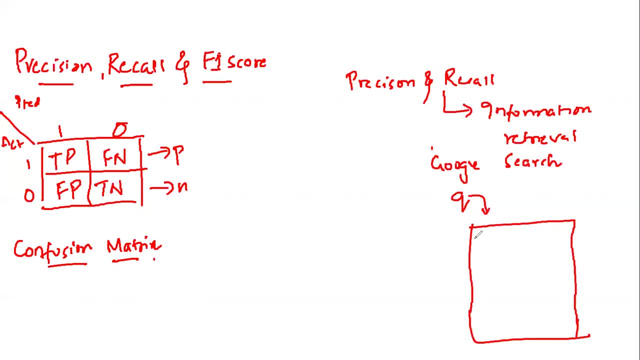 a million of records. right Based on this query, we may be having a million of records And from this million of records the top, most relevant records will be actually retrieved. So this precision recall is very, very important in information retrieval. So, considering this, 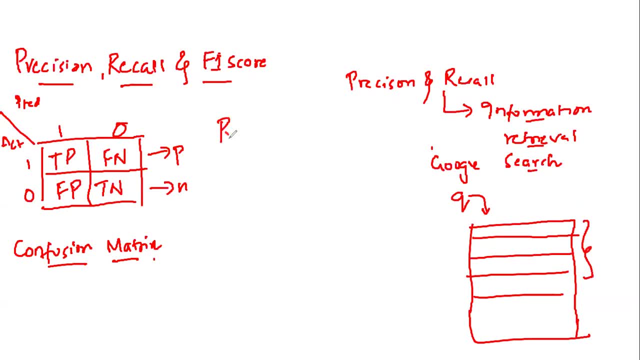 particular fact. let me define the precision formula. So precision is basically given by true positive divided by true positive plus false positive. Now, many of them will get confused with this particular equation, but let me just write it down in simple words. This basically says that out of the total, out of the total, 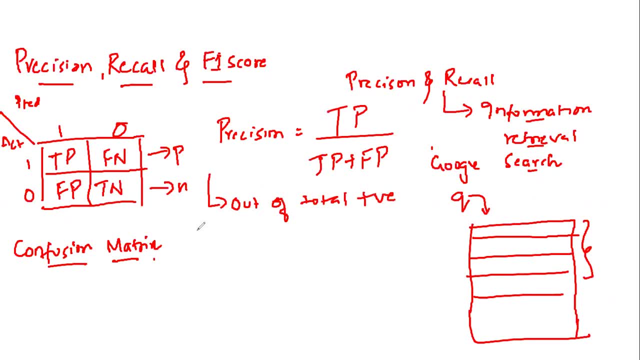 precision basically says that, out of the total positive predicted results by the model, out of the total positive predicted results, TP is basically the positive results, right? So out of the total positive results that are predicted by the model, what is the what? 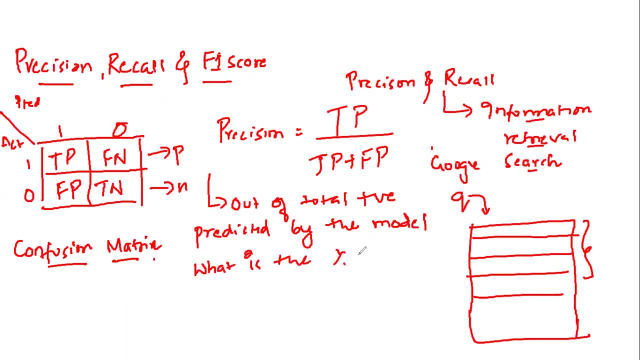 is the? what is the percentage of actual positive result? The equation basically specifies that. the precision basically specifies that, out of the total positive results, out of the total predicted positive results. Now, if I go and see TP and SP right, These are: 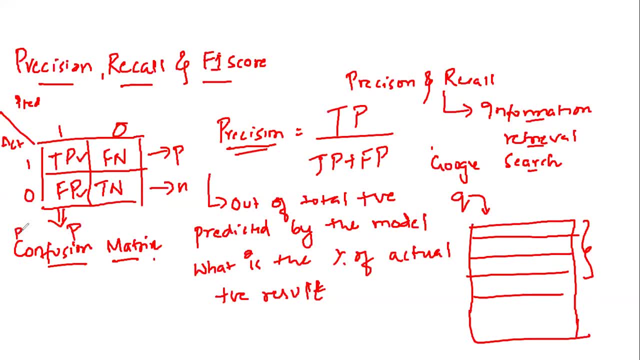 the total number of positive predicted results. right, So these are my total positive predicted results. So from this, from this, from this, it is telling that how much is my TP, or what percentage is basically my TP. And if I said TP, TP, so this TP is nothing, but it is nothing. 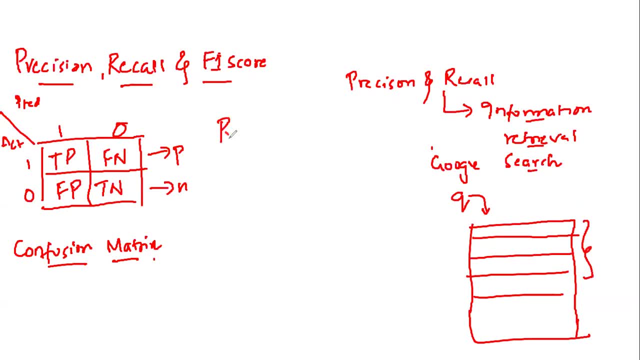 particular fact. let me define the precision formula. So precision is basically given by true positive divided by true positive plus false positive. Now, many of them will get confused with this particular equation, but let me just write it down in simple words. This basically says that out of the total, out of the total, 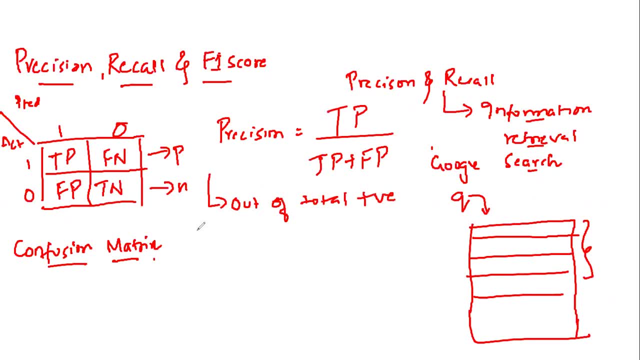 precision basically says that, out of the total positive predicted results by the model, out of the total positive predicted results, TP is basically the positive results, right? So out of the total positive results that are predicted by the model, what is the what? 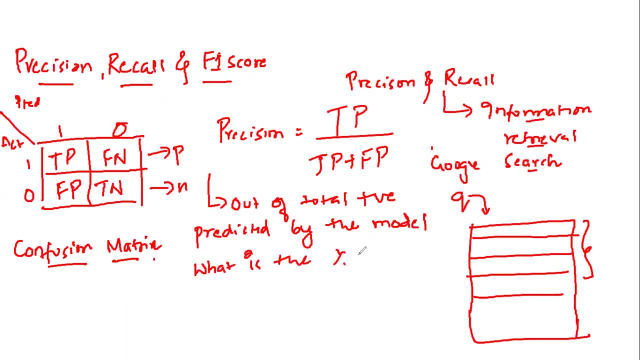 is the? what is the percentage of actual positive result? The equation basically specifies that. the precision basically specifies that, out of the total positive results, out of the total predicted positive results. Now, if I go and see TP and SP right, These are: 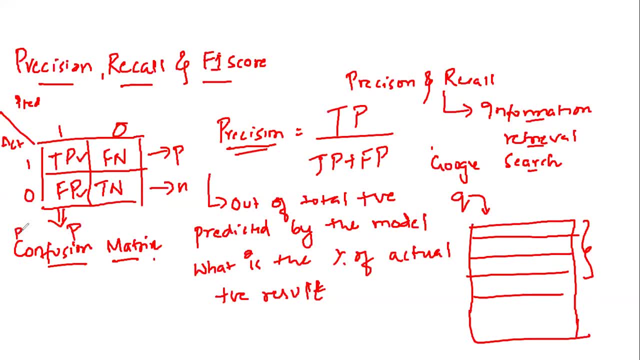 the total number of positive predicted results. right, So these are my total positive predicted results. So from this, from this, from this, it is telling that how much is my TP, or what percentage is basically my TP. And if I said TP, TP, so this TP is nothing, but it is nothing. 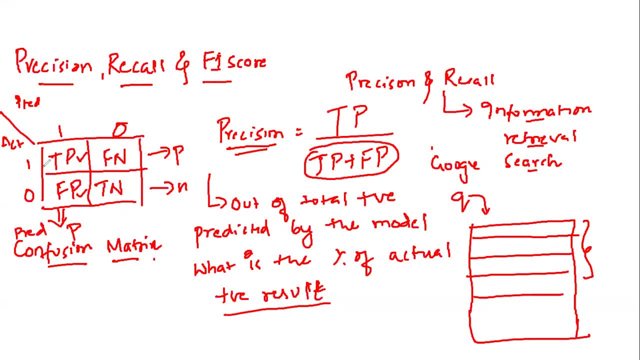 but the percentage of actual positive results. right, So it is the percentage of actual positive results. So this is how precision is basically defined. Now, guys, you may be considering why True positive? because just understand if I, if I told you that now, now we have already. 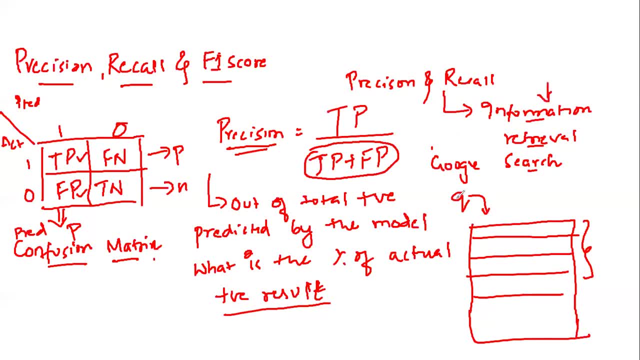 seen that precision and recall are basically useful information retrieval right And whenever in Google search engine we write a query, we try to retrieve the most relevant records. So these are the most positive. you know positive records that I have gone because 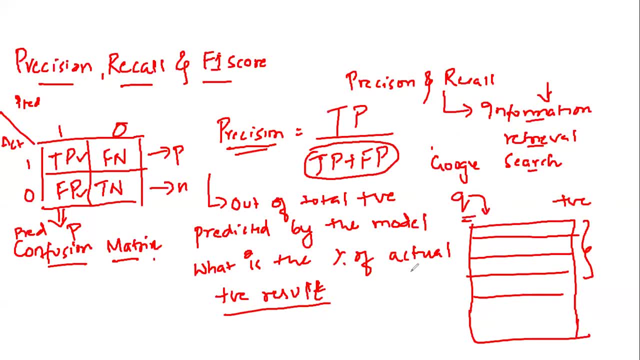 that is completely based on the relevance of this particular query right. So these are the most relevant records that I want with respect to this particular query. So precision recall: Basically you know they work on only positive results. Positive result basically means that 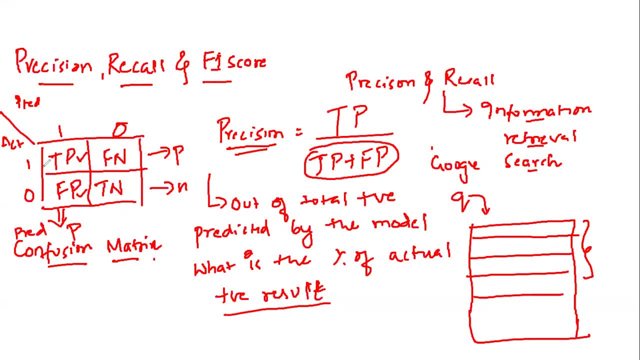 but the percentage of actual positive results. right, So it is the percentage of actual positive results. So this is how precision is basically defined. Now, guys, you may be considering why True positive? because just understand if I, if I told you that now, now we have already. 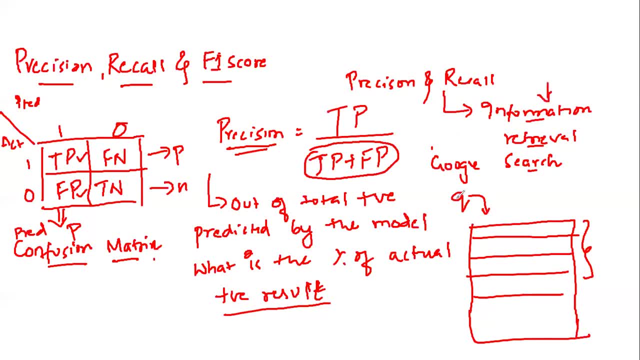 seen that precision and recall are basically useful information retrieval right And whenever in Google search engine we write a query, we try to retrieve the most relevant records. So these are the most positive. you know positive records that I have gone because 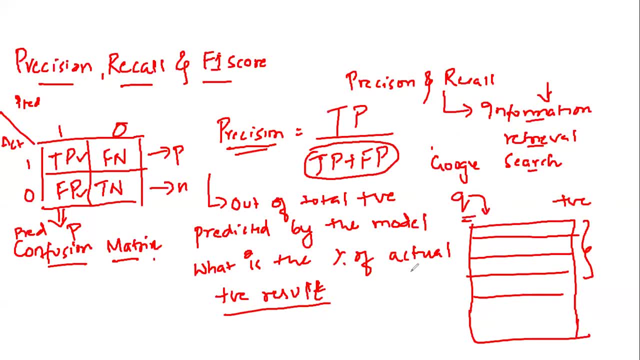 that is completely based on the relevance of this particular query right. So these are the most relevant records that I want with respect to this particular query. So precision recall: Basically you know they work on only positive results. Positive result basically means that 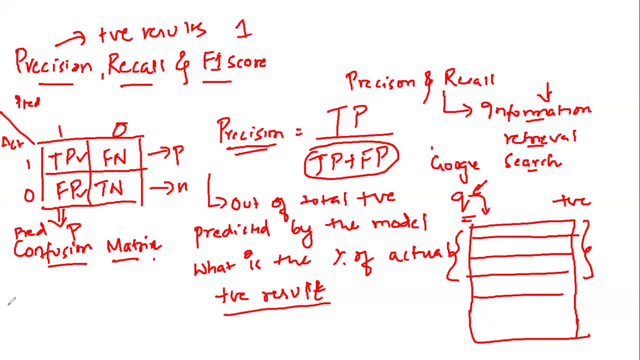 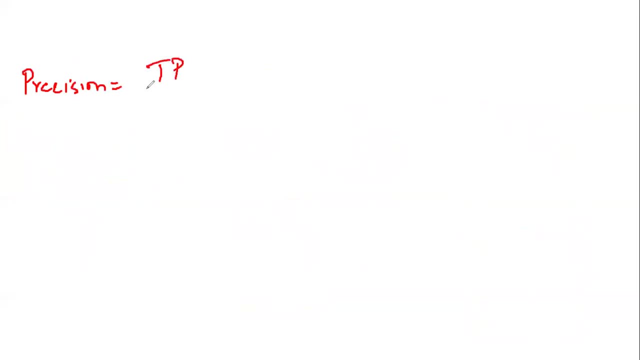 in this case, is basically one: Yeah. Now, the next thing is that what is recall? Okay, So I'm just going to again write this down. equation: completely: Okay, So precision is nothing, but I'll write. just write it down as decision is nothing but TP divided by EP plus F, Right, 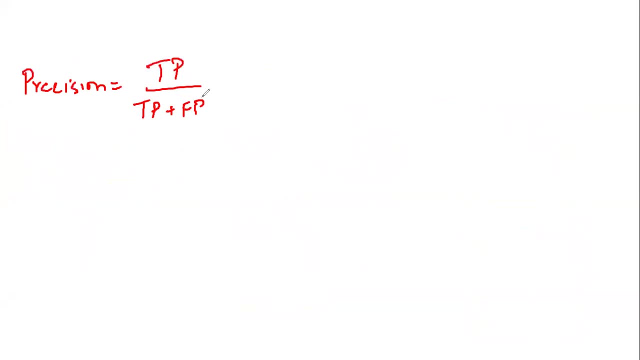 And I've also told you that out of the total, you know the percentage of actual positive predicted results. what is the percentage of the actual positive results? So that is what precision says. Recall is nothing, but it is basically given by. it is same as true. 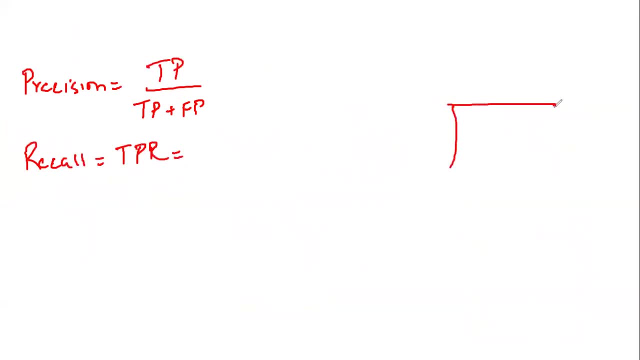 positive rate. Now, if you remember true positive rate, I'll just draw a confusion matrix again. Okay, This is my predicted value. This is my actual value. Now, here I have one zero. here I have one zero. now two positive rate. What is two positive? It suppose this is my. 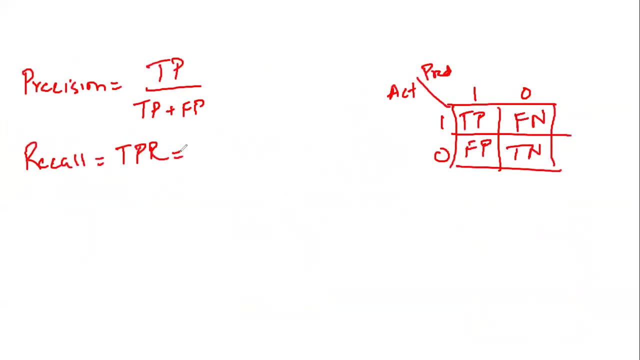 true positive, true negative, false negative and false positive. true positive rate is nothing but tp divided by the total number of actual positive results. what are my total number of actual positive results, which is nothing but this p, and this is basically total number of actual negative results. so again, why i am considering recall for tpr, not as tnr, because we are just 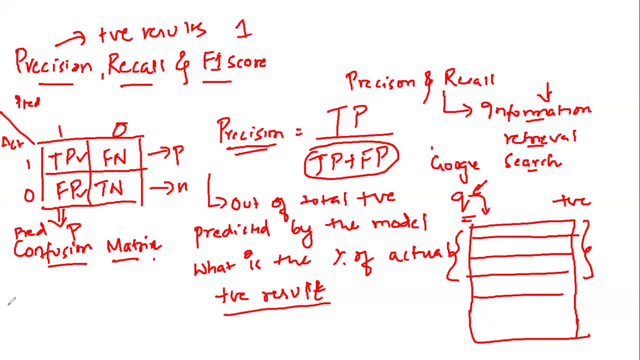 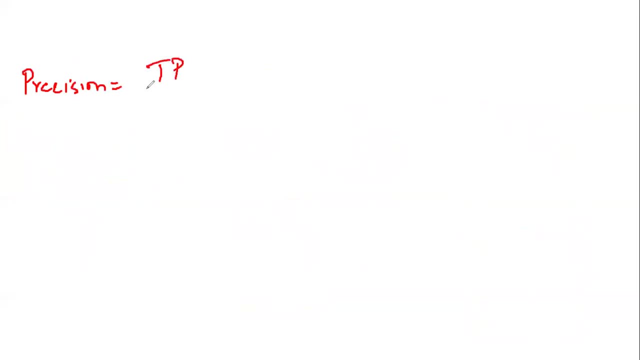 in this case, is basically one: Yeah. Now, the next thing is that what is recall? Okay, So I'm just going to again write this down. equation: completely: Okay, So precision is nothing, but I'll write. just write it down as decision is nothing but TP divided by EP plus F, Right, 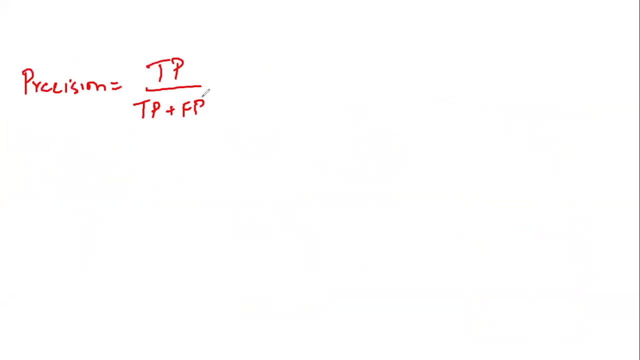 And I've also told you that out of the total, you know the percentage of actual positive predicted results. what is the percentage of the actual positive results? So that is what the season says. Recall is nothing, but it is basically given by. it is same as true. 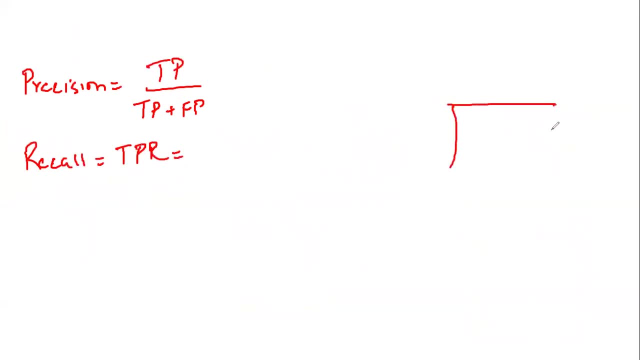 positive rate. Now, if you remember true positive rate, I'll just draw a confusion matrix again. Okay, This is my predicted value. This is my actual value. Now, here I have one zero. here I have one zero. now, true positive rate. What is true positive rate? Suppose this is. 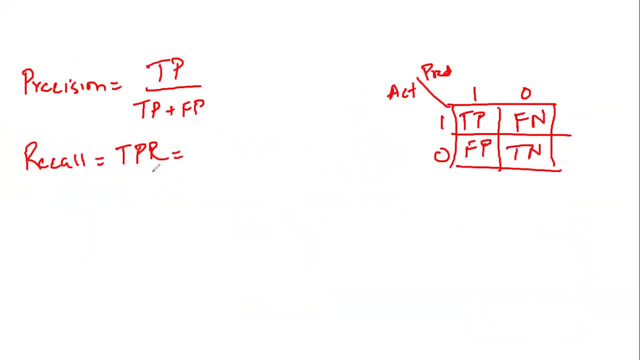 my true positive, true negative, false negative and false positive. True positive rate is nothing but TP divided by the total number of actual positive results. what are my total number of actual positive results, which is nothing but this peak, and this is basically. 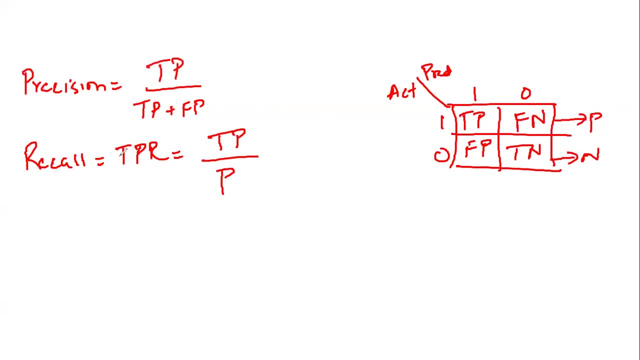 total number of actual negative results. So again, why I'm considering the call for TPA are not as TNR, because we are just focusing the precision recall are mostly calculated for, you know, one and zeros. Sorry, once, only for once. Now suppose if I want to calculate for my negative number, then suppose I want to calculate. 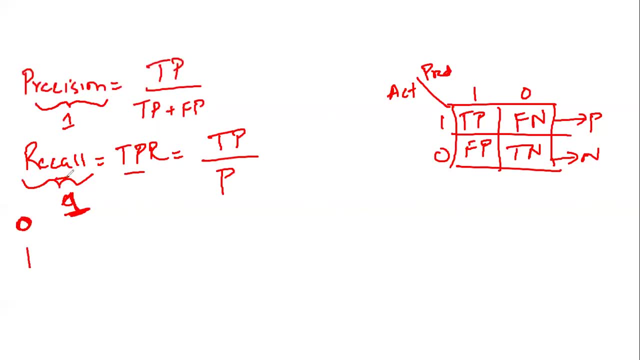 for my zero, my net false. uh, false value. Okay, Currently I'm just, you know, I'm calculating for one. I can also calculate for non relevant results. So far, zeros. how my precision by equation will get changed is nothing, but I can write it as true. negative to negative. 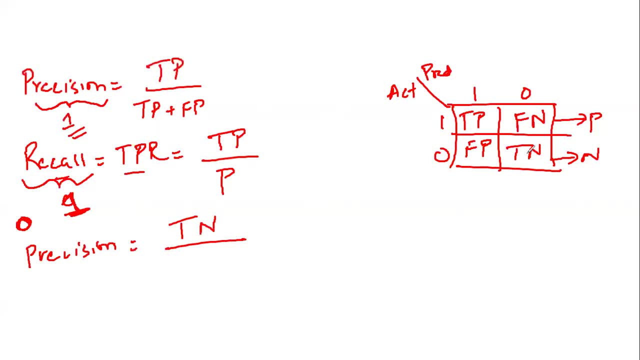 divided by- uh sorry, true negative. divided by the total number of predicted negative values. So I can write it as DN, by FM. So this is how I will be writing my precision. Now, what does this say? that out of the, out of the total, total negative results negative. 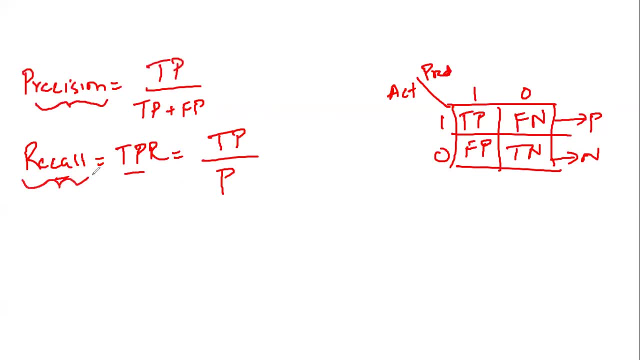 focusing the precision recall are mostly calculated for, you know, one and zeros. sorry once, only for once. that is my positive one. now suppose, if i want to calculate for my negative number, then suppose i want to calculate for my zero, my next false, uh, false value, okay, currently. 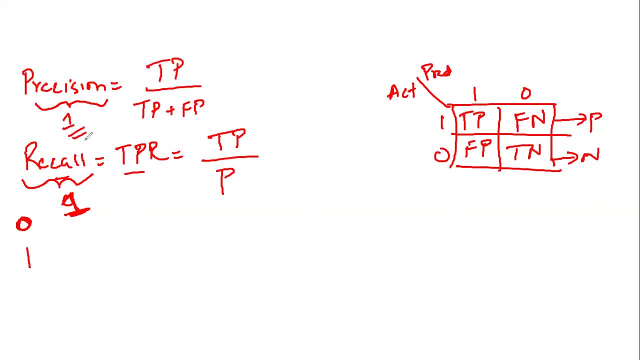 i'm just, you know um calculating for one. i can also calculate for non-relevant results also. so for zeros, how? my precision where equation will get changed is nothing. but i can write it as true negative. true negative divided by- uh sorry, true negative divided by the total number of predicted negative values. so i can write it as tn by fm. 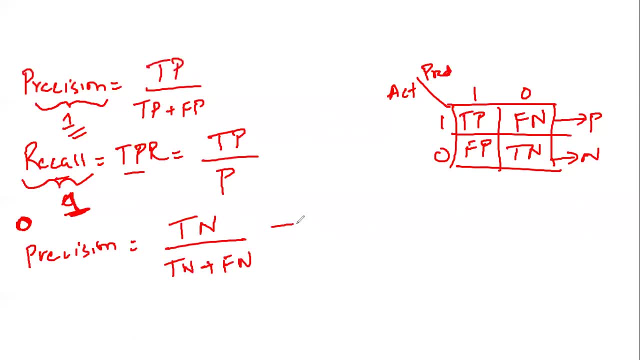 so this is how i will be writing my precision now. what does this say? that out of the out of the total total negative results, negative correct results that were predicted. okay, so these are my total negative results, right? what is the percentage of the negative value? the actual negative value? actual negative value. so this is what that particular value specifies. 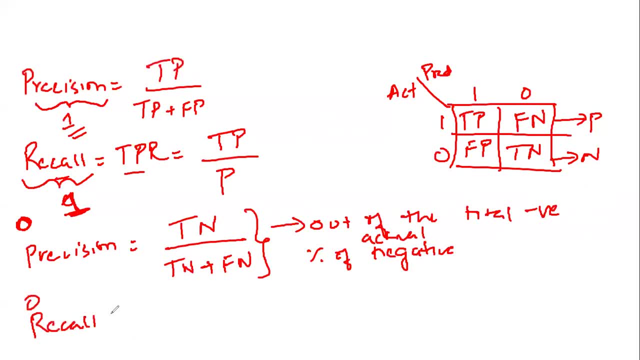 okay, and similarly for the zero value, the recall can is nothing, but it is similar to, uh, something called as true negative rate. right, and we know that true negative rate is nothing but true negative divided by the total number of negative results. and this is how you- you actually use this precision and recall with respect to your one. 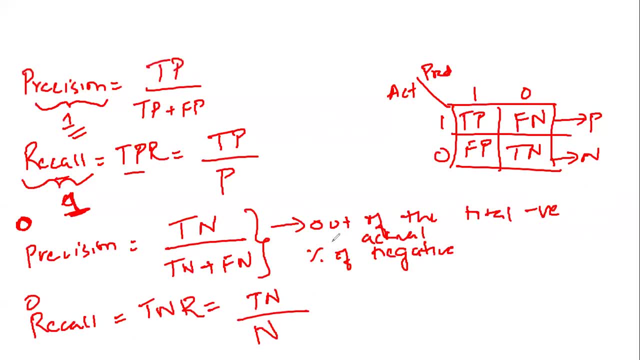 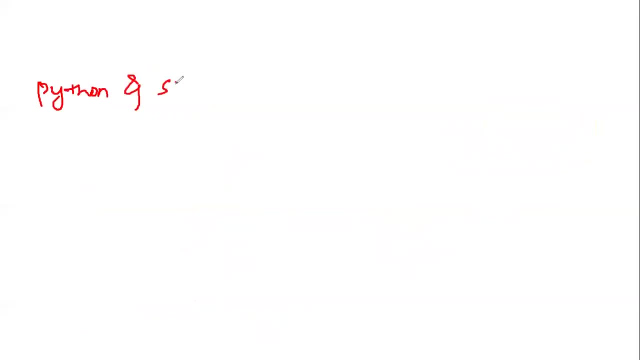 value and with respect to your zero. so we have an option to get both this particular value, and this is how the formula is basically designed. now the next thing is that some may be thinking that how can we implement this by using python? by using python and a scalar right, how can we implement? 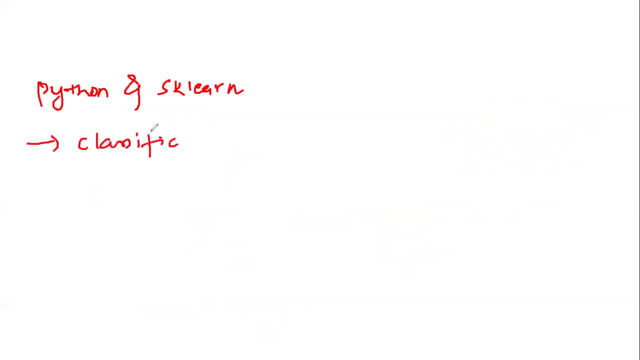 so we have a library which is called as classification classification underscore report. in this classification underscore report we just give our y predicted uh as my parameter, as y uh, the y test value. so why real taste value and the y predicted value? as soon as i give this with respect to one zeros. 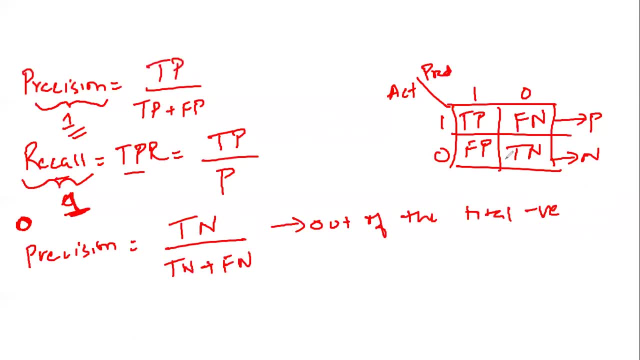 correct results that were predicted. Okay, So these are my total negative results, right? What is the percentage of the negative value? the actual negative value, actual negative value. So this is what that particular value specifies. Okay, And similarly for the net zero value. 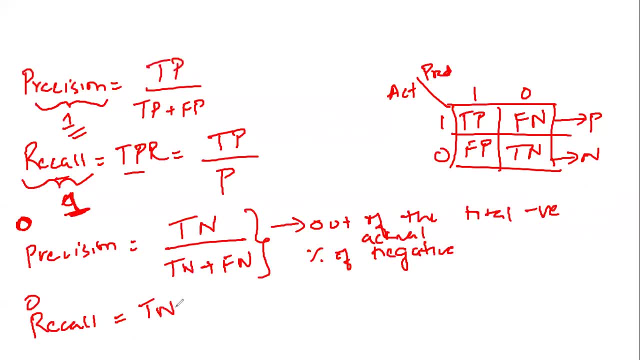 the recall can is nothing, but it is similar to, uh, something called as true negative rate. Right, And we know that true negative rate is nothing but true negative divided by the total number of negative results. And this is how you, you actually use this. 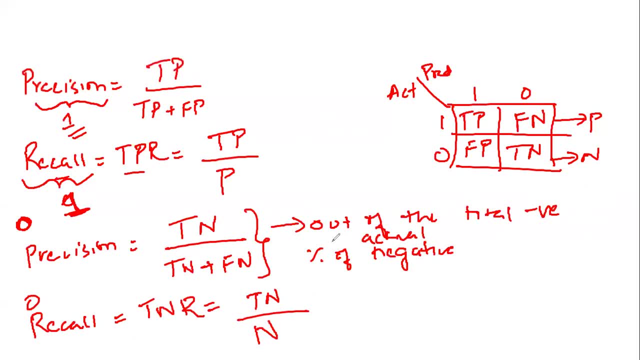 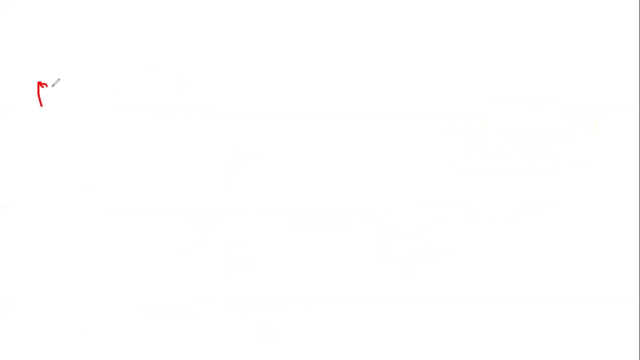 precision and recall with respect to your one value and with respect to your zero. So we have an option to get both- this particular value, And this is how the formula is Now. the next thing is that some may be thinking that how can we implement this by using Python. 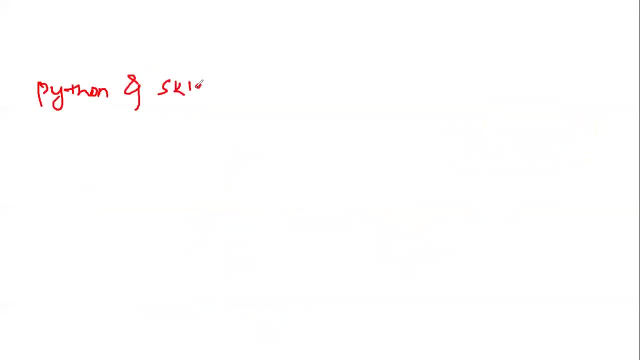 by using Python and a scale of right. How can we implement? So we have a library which is called as classification classification underscore report. In this classification underscore report, we just give our why predicted uh as my parameter. as why, uh, the white test value. So why real test value and the white predicted? 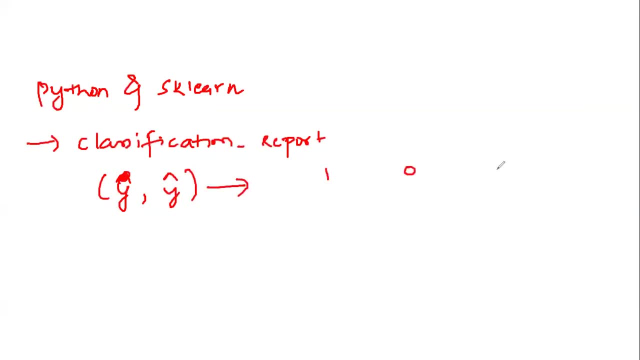 value. As soon as I give this with respect to one zeros, right, I'll be getting what is my precision, What is my recall, Okay, And based on this, I will be basically getting the value between, you know, one zero to one, and this can be converted into percentage. 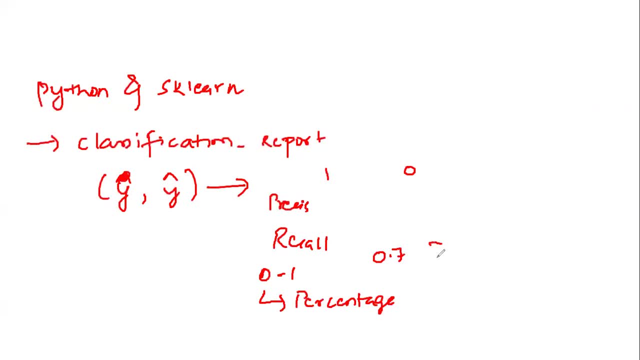 This can be converted into percentage. Suppose, if I'm getting 0.7,, this is nothing but 70%. Now, the next thing is that I will try to combine precision and recall recall together with the new measure which is called as F1 score. Now, F1 score is basically given as two multiplied. 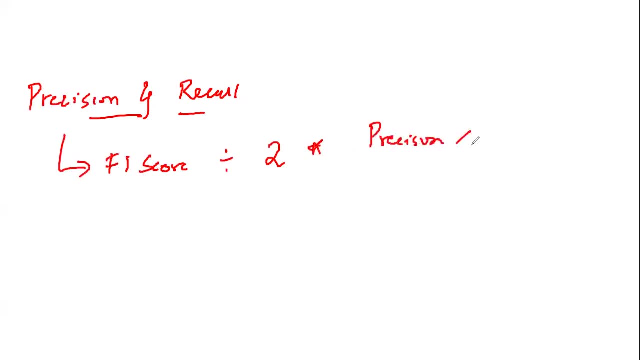 by precision into recall divided by Okay, So precision plus recall. And again, when I'm calculating F1 score, I can calculate separately for one and I can calculate separately for zero, because for one and zeros I may have different, different precision and recall. Again, note guys, this value will be between: